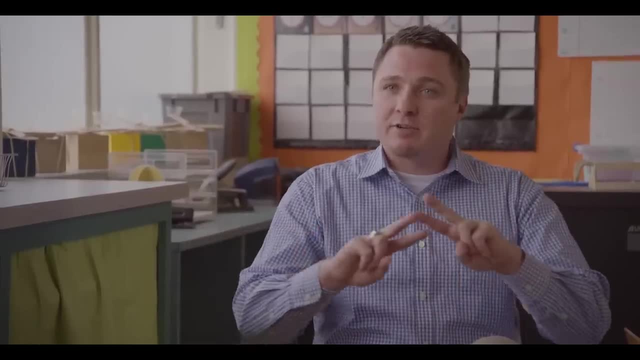 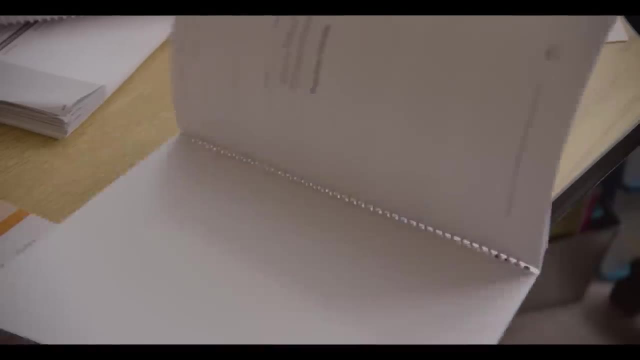 the year. Instead of teaching things in isolation, it's teaching a lot of different concepts at the same time, And when we came across CKLA, it wasn't presented with a big sales pitch, There weren't a lot of bells and whistles, It was just pretty straightforward. Here's a program that can. 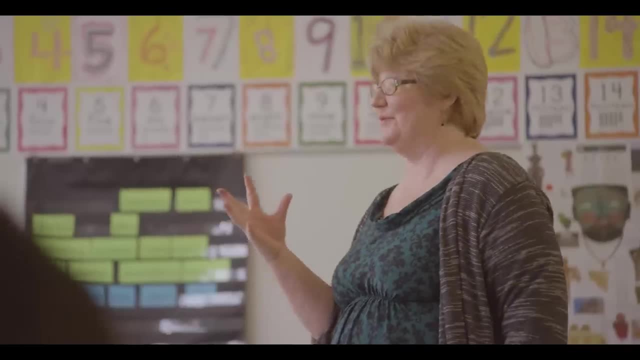 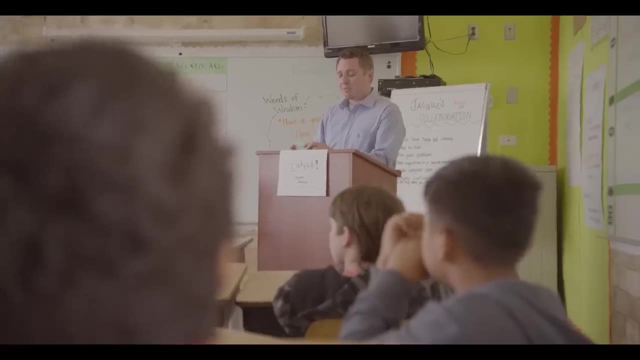 address foundational skills. it's got a content, knowledge and it's going to work for your EL students as well. I think the bottom line is: after all the years of seeing language arts programs that are very similar, this has been a huge change: Their support in helping us out in training. 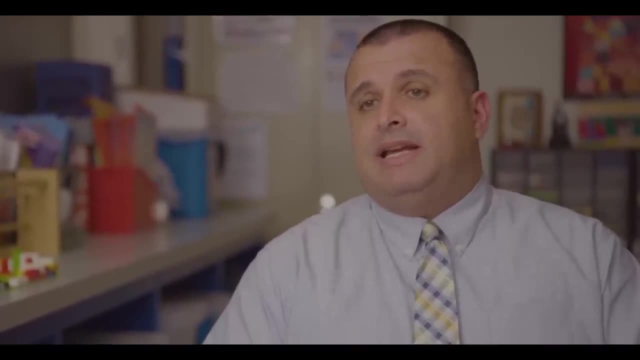 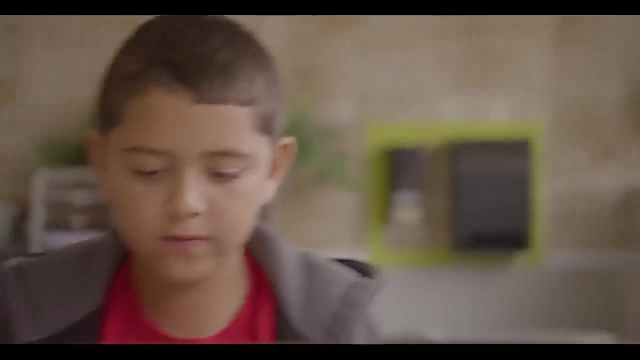 our teachers and making sure that the curriculum was used appropriately was just second to none. I was really doubtful in the beginning As a teacher. it was terrifying. I thought: how is this going to work? They say that it will. I can see that it might, but I'm not sure. 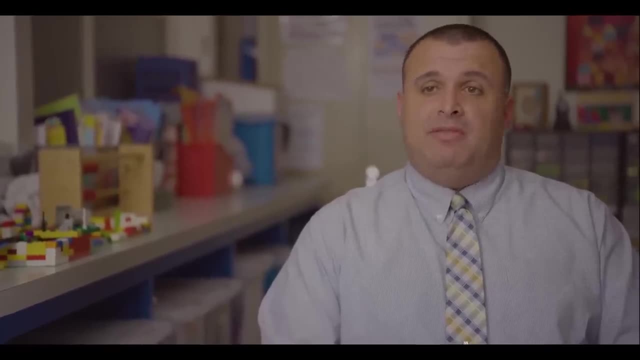 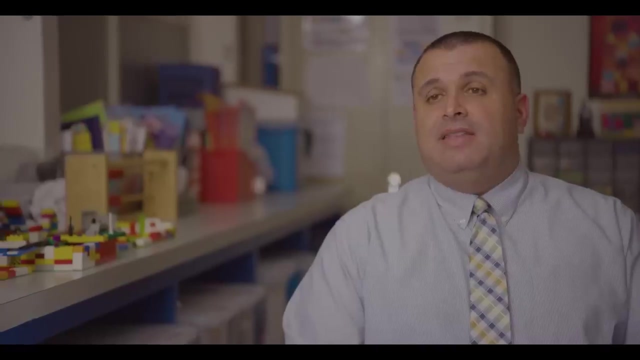 I felt like we underestimated our kids. Amplify does hold a lot of rigor and we, for a second. when we started this program, we felt that kids were not going to be able to meet those expectations. And they have. They surpassed it and we are seeing tremendous amounts of 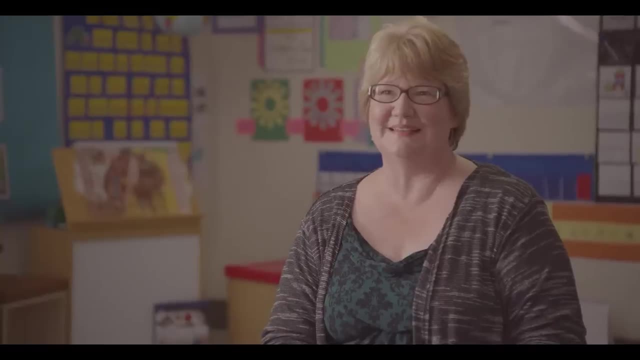 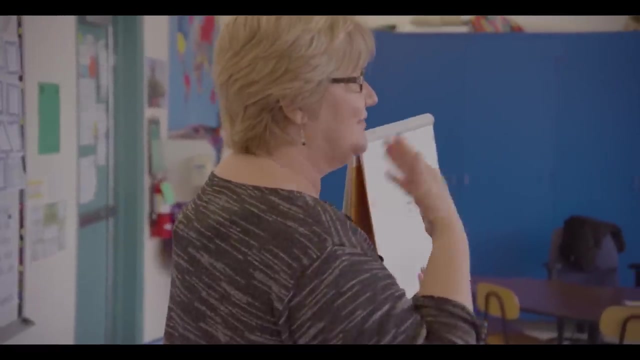 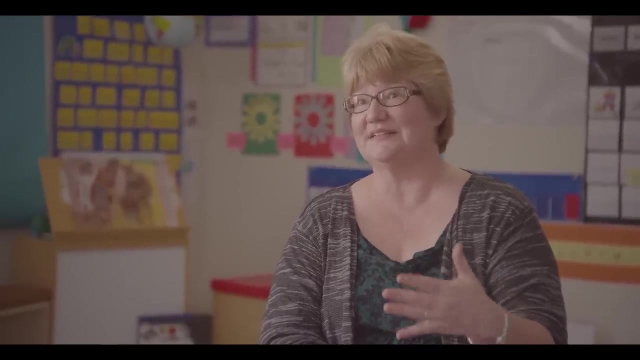 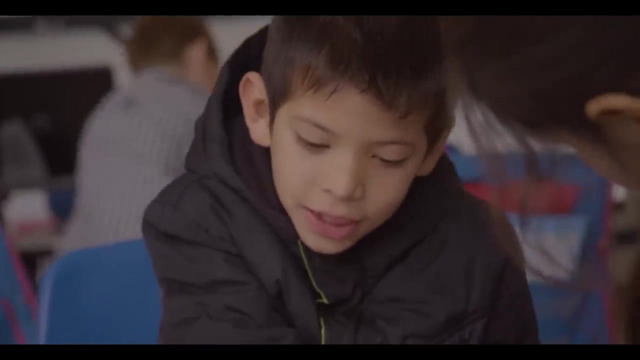 growth. They are reading things that typically we wouldn't be reading Reading this early in the year. Very good, The sound is ow. Everyone say ow, Ow. The introduction of the sounds follows a very different sequence than any other program I have used in the past. The kids seem to be picking it up more quickly. 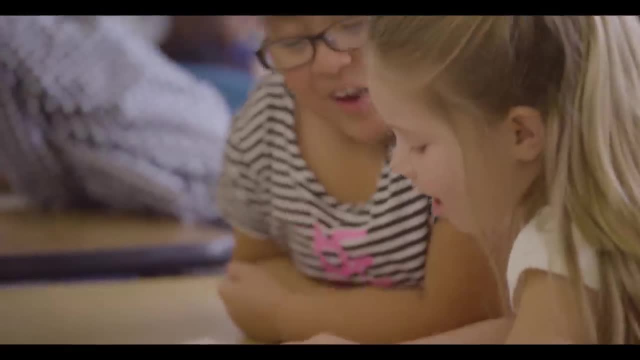 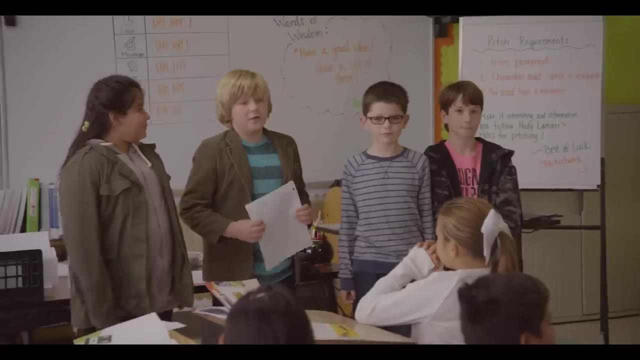 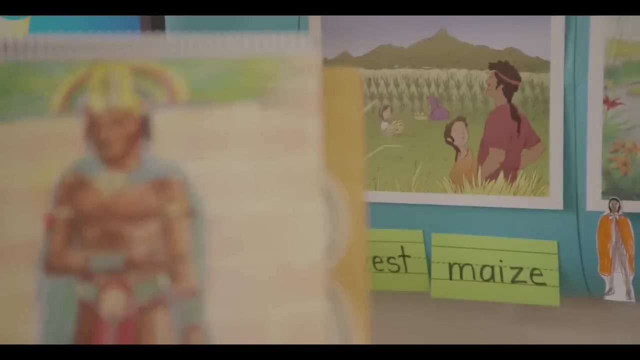 Once a man went up. Major differences that I am seeing are the ability of my students to communicate to each other. Hello, fellow classmates. I'm here today to talk about the invention of the clock. The inclusion of the knowledge piece is so important, And I think that is the one thing. 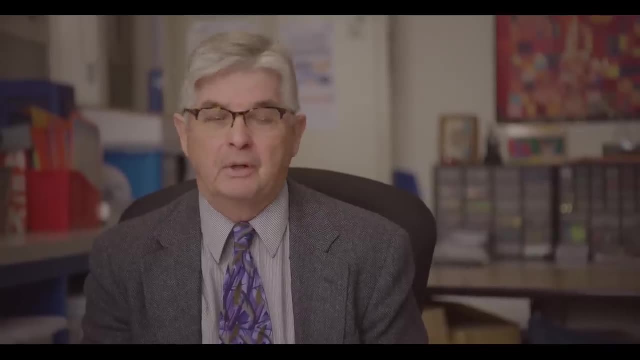 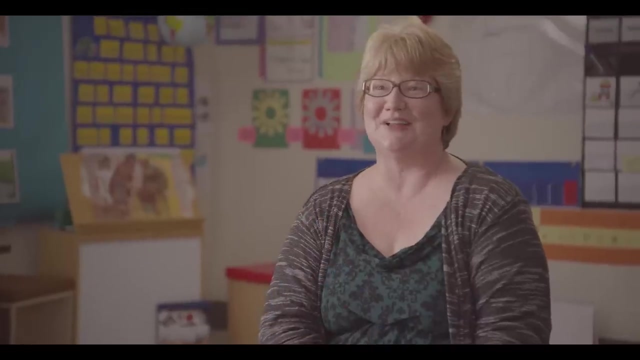 that we are really finding the payoff. Kids are reading about something and they are responding, And the responses that they are writing are head and shoulders above where they were before. My favorite part is the knowledge piece. because of the storytelling, because of the interests, Later, Montezuma and his chief advisors met together. Very cool. How did you two meet? Very interesting, very interesting, Very interesting. So what was the difference? Very interesting, very interesting, Very interesting. What was it like when you and the kids met? 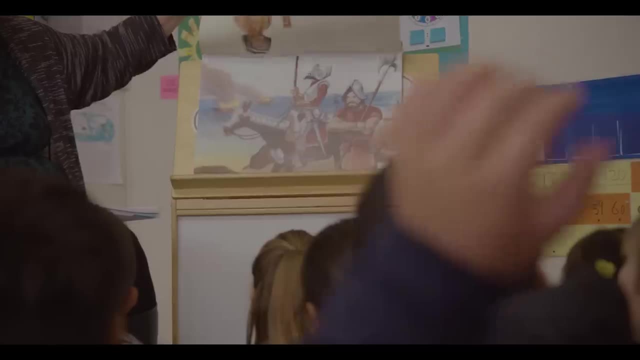 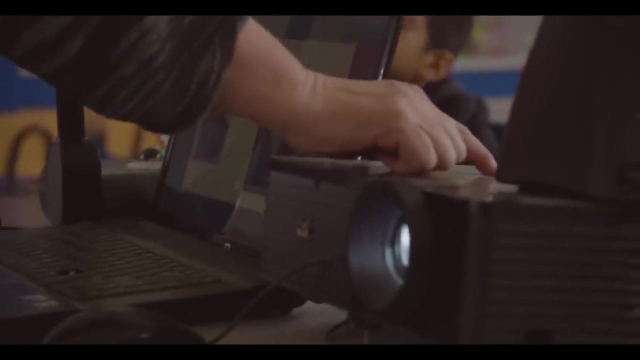 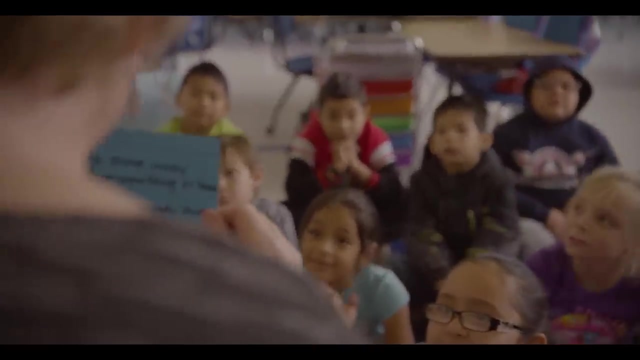 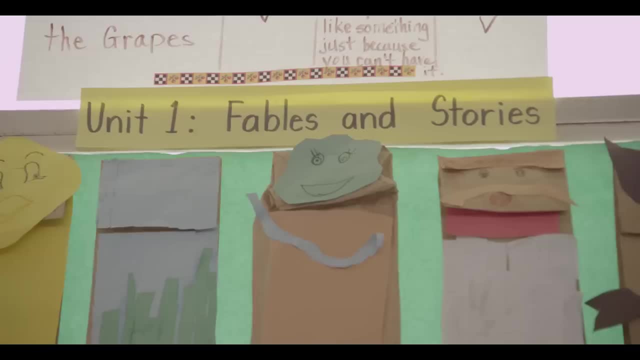 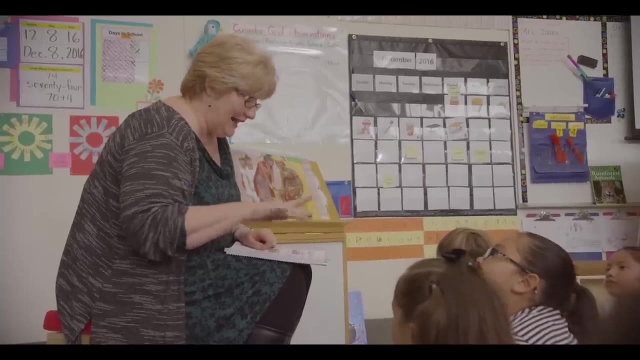 Core Knowledge. it helped bring the learning alive. in learning the language components. It wasn't just rote skills of grammar or vocabulary, It was actually tied to something that was you know worldly. It meant something in their lives. What is a pitch? 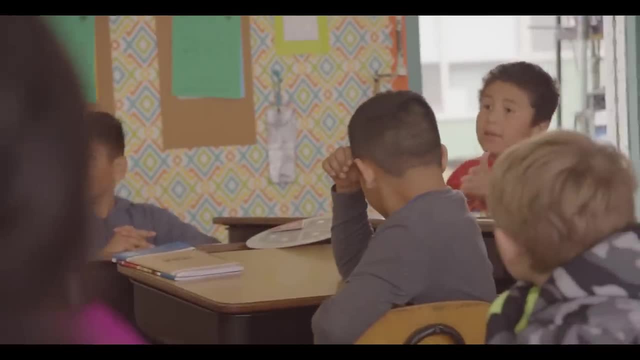 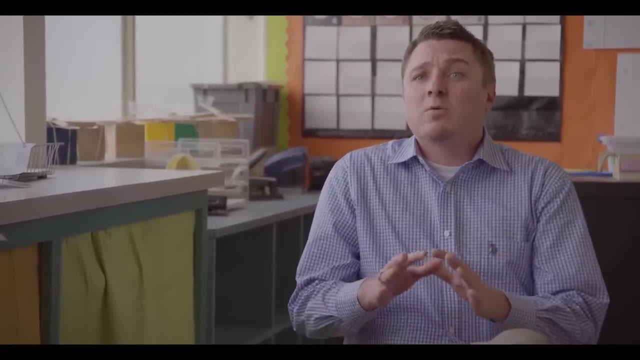 There's a good pitch and a bad pitch If a good pitch is, like many facts, well organized, informative. They're learning about lords and serfs and they were comparing and contrasting without even knowing that they were comparing and contrasting. What I like about CKLA is that 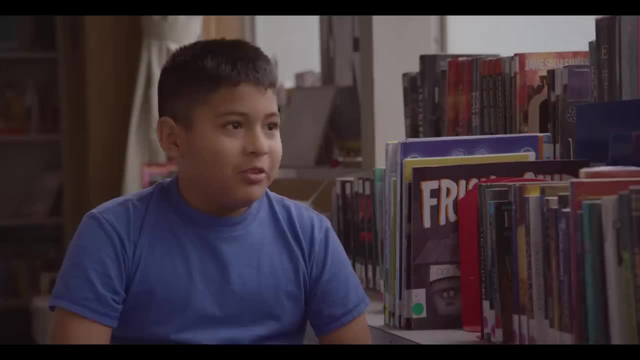 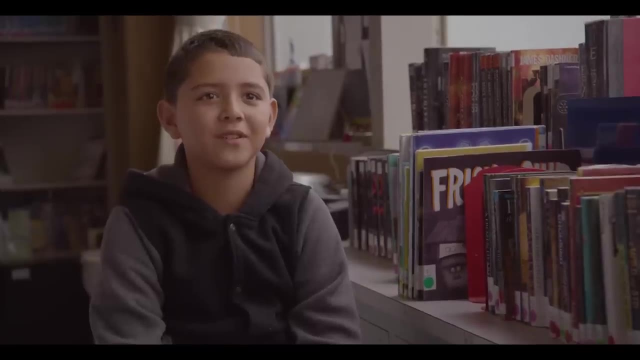 we get to learn about all the inventors and do research on them. It's basically science and experiments and history- Only one bunch. Really cool. It's a lot more fun this year with CKLA. Okay, guys, welcome back to today's episode of. 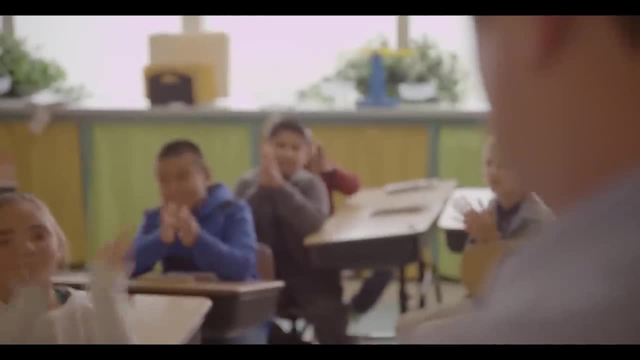 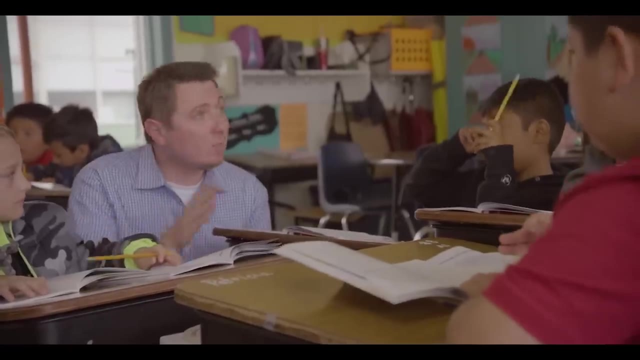 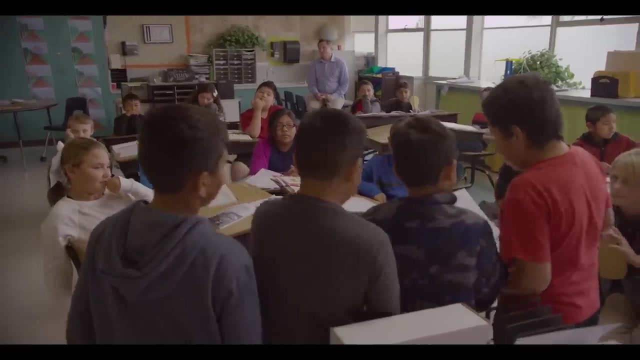 Eureka. As a teacher, I've learned a lot from CKLA. There are times when I'm looking at a lesson and I will kind of look and think that's amazing. The way that they were able to teach that specific skill in many ways was ingenious. The map that they have is unparalleled, So is there a specific? 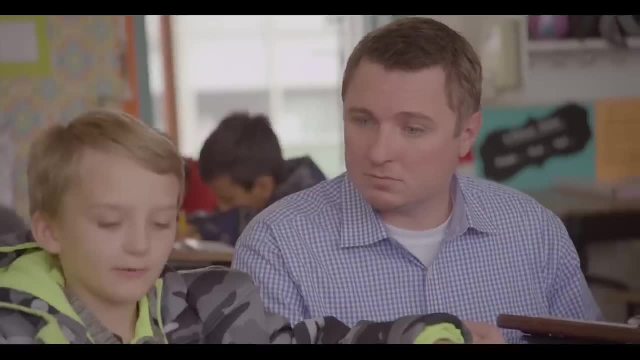 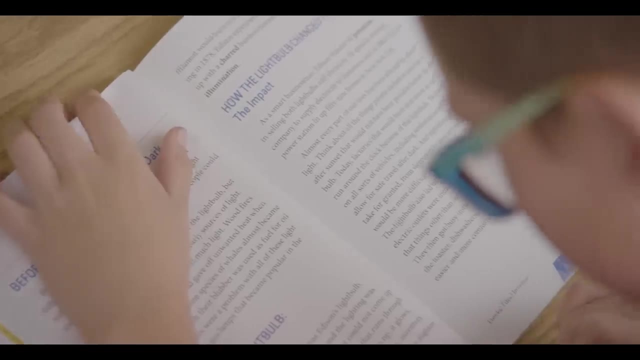 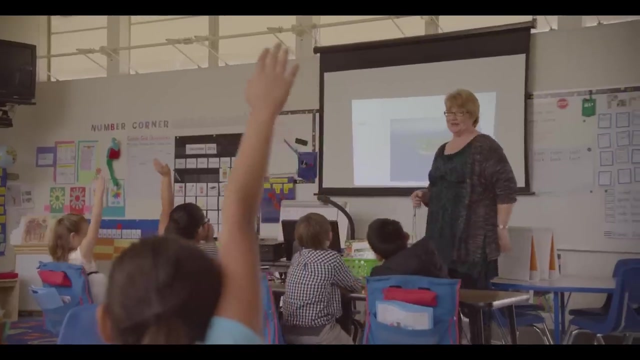 information. Yeah, Which one? It would have to be lessons in Russian. We certainly like to see the way the program spirals throughout the year within a grade level. The spiraling between grade levels is really neat, The fact that kids are going to see something in first grade and third grade and 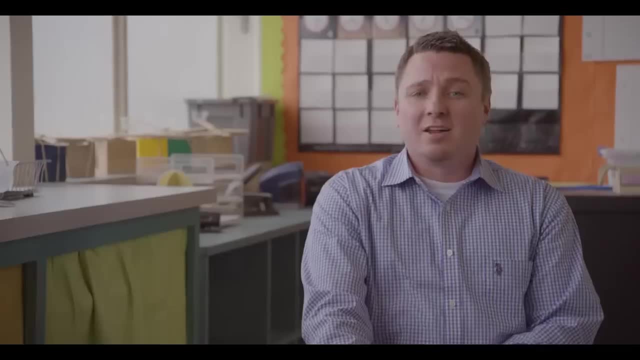 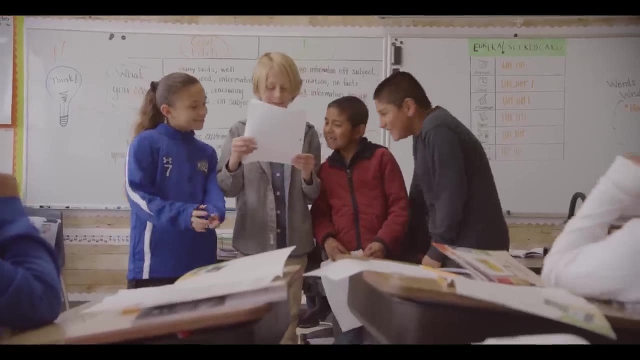 fifth grade. it's just going to reinforce their love for learning it. Lots of times the bell will ring and they want to continue. just let us finish. just let us finish. give us five more minutes. The fact that we have a curriculum that compete with recess, that's a huge deal. Yeah, it goes by very quickly.